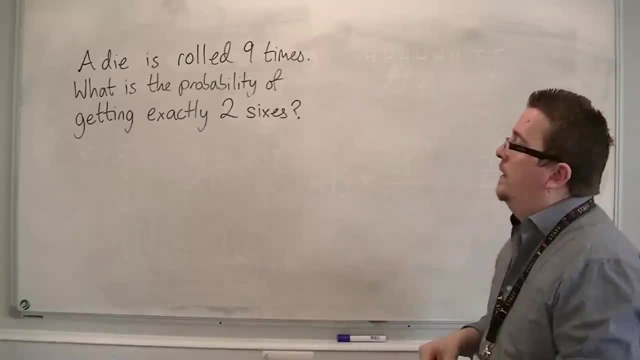 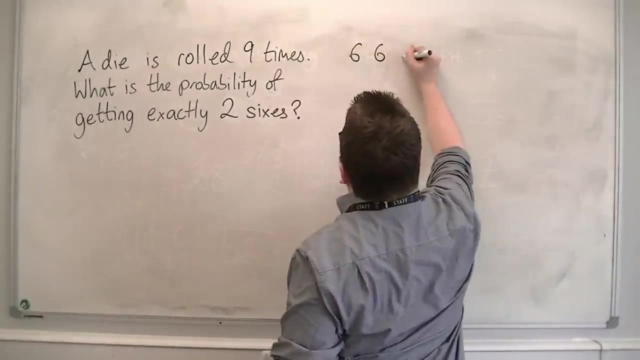 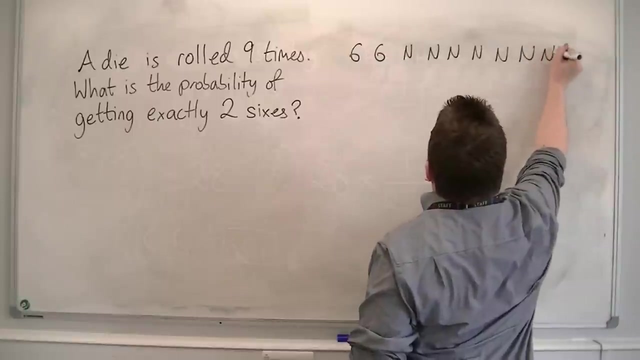 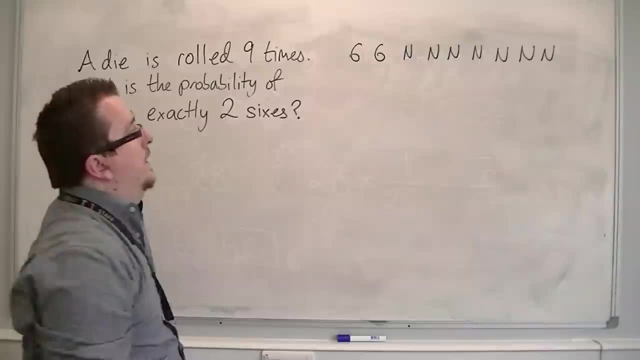 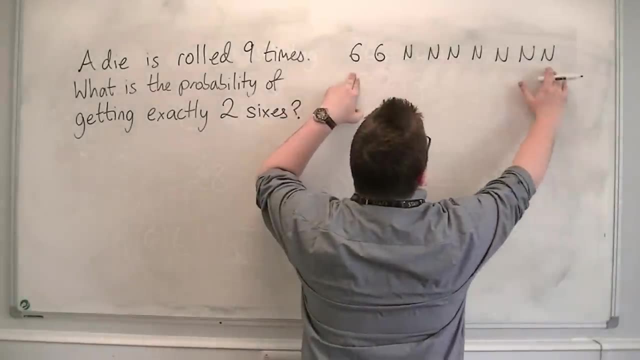 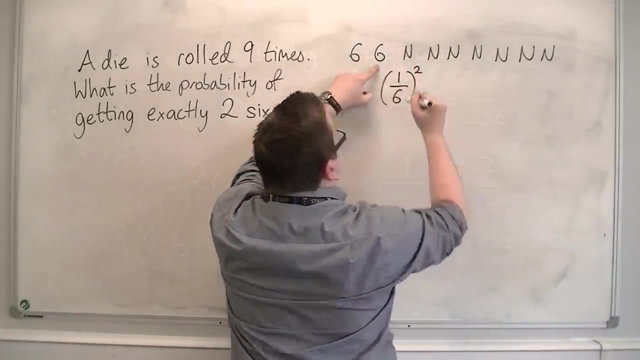 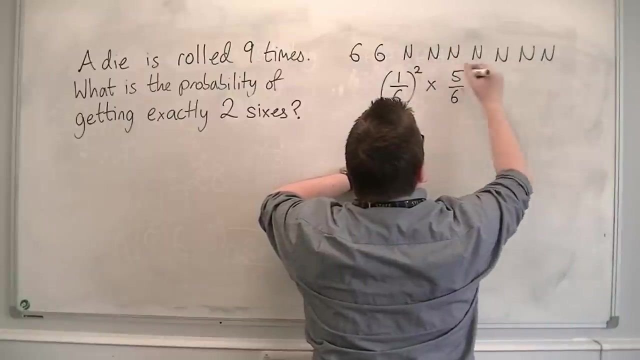 One, two, three, four, five, six, seven, eight, nine. So that is one of the possibilities. Now to work out the probability of that. well, this is one over six times one over six. so one over six, squared times five over six. one, two, three, four, five, six, seven. so to the power of seven. 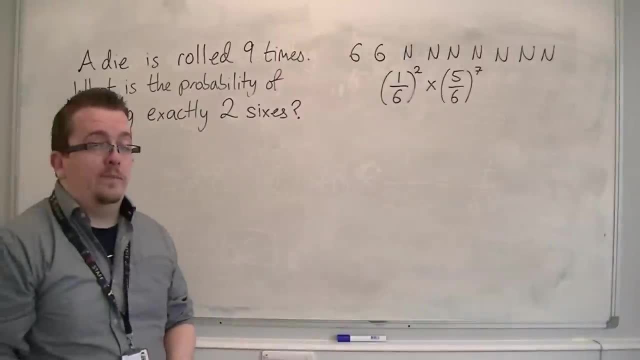 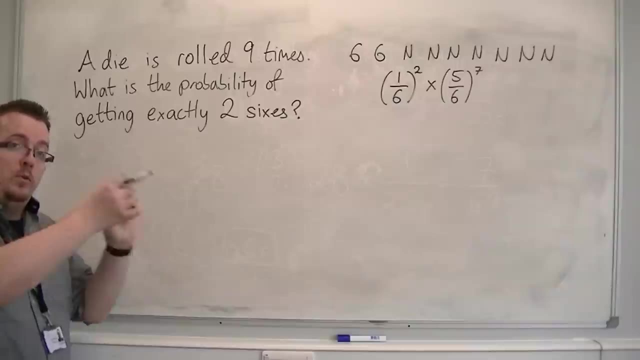 So one over six, squared times five over six. So that's the probability of just one of the events occurring. But there are going to be multiple combinations, multiple ways of doing it. So if I want, out of a possible nine to get two sixes, then I want to find nine NCR two. 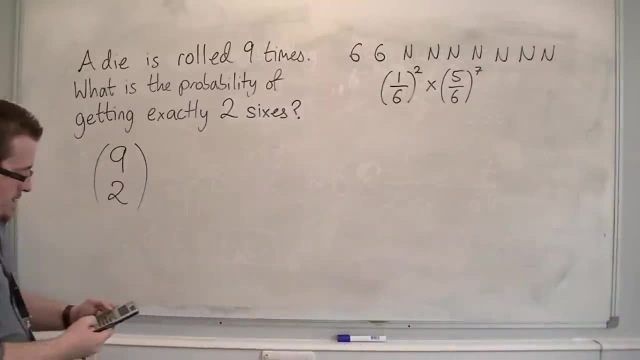 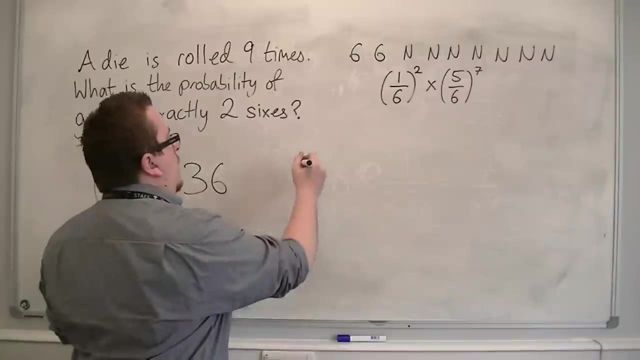 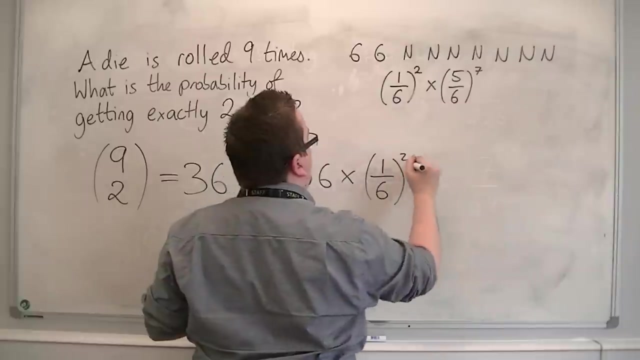 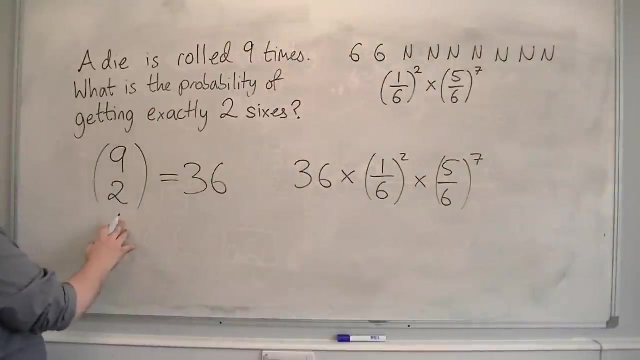 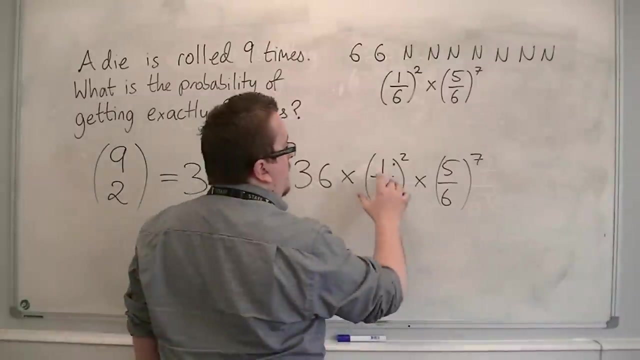 OK, so I find nine NCR two on the calculator, and that gets me 36.. And so the probability for this question is 36 times one over six, squared times five over six to the seven. So it's the number of possible combinations times by the probability of the event occurring, by how many times I want it to occur, times the probability of it not occurring, to the power of how many times it won't show up. 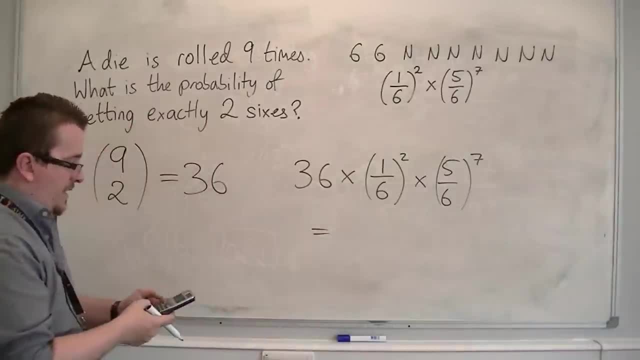 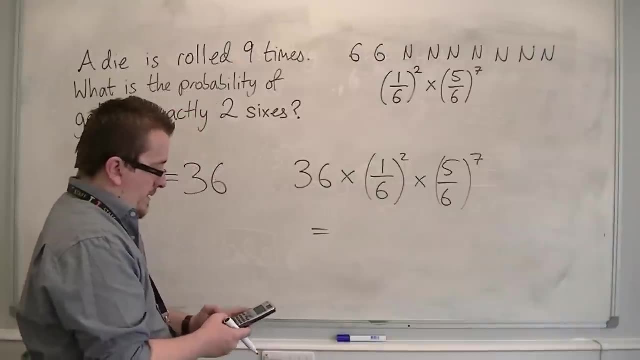 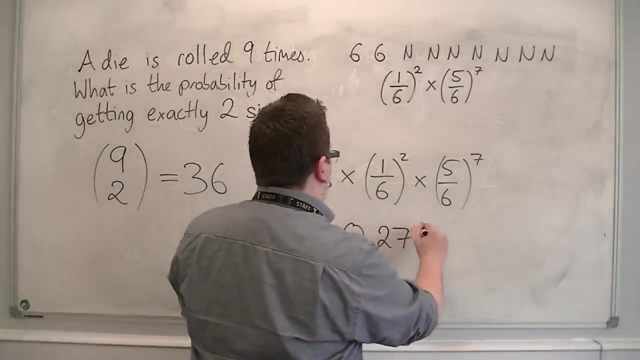 Well, we don't want it to show up, So I plug that into the calculator: 36 times one over six squared, and then you're going to times that by five, sixths to the power of seven, And that gets me 0.279 to three significant figures. 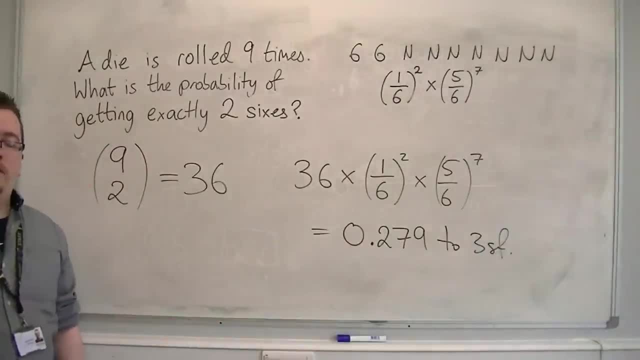 OK, and that's how we can deal with unequal probabilities like this.